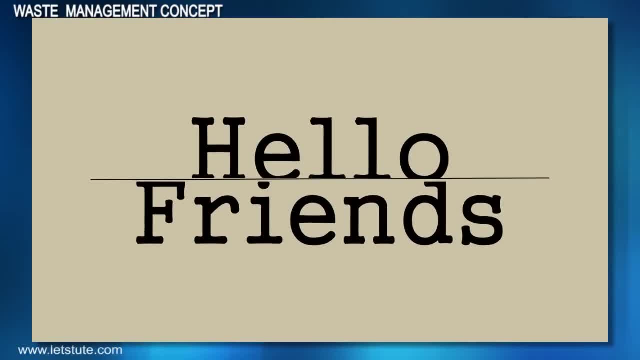 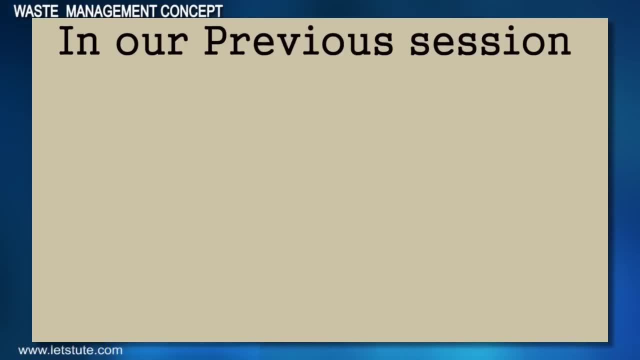 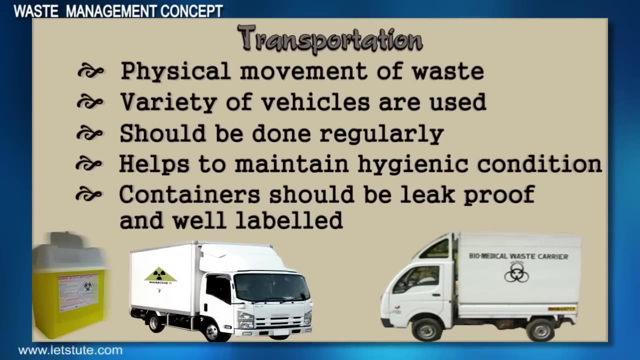 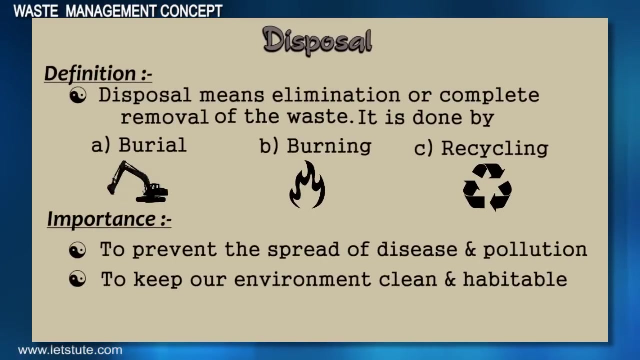 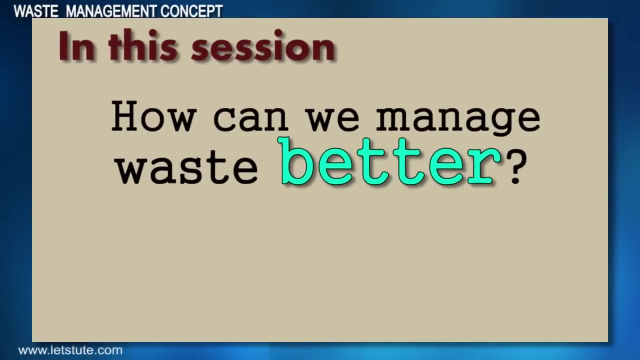 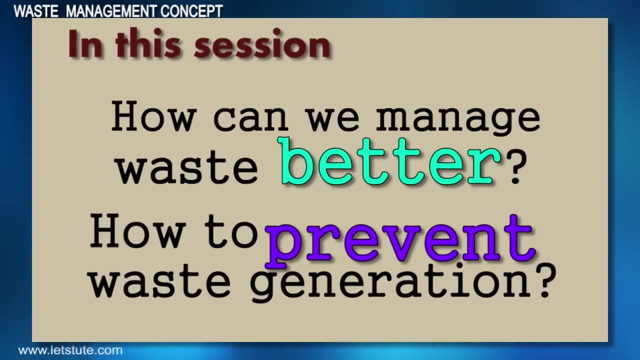 Hello friends, here we are with yet another session on waste management. Previously, we learnt about all the various steps involved in waste management, focusing mainly on transportation, treatment and disposal of the waste, And, as promised, today we'll know the various ways to manage waste better, which will also help us in reducing the very generation of waste. Yes, my friends, it is the principle of 7 R's. 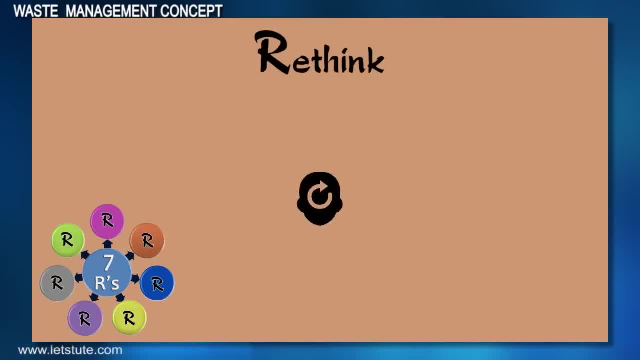 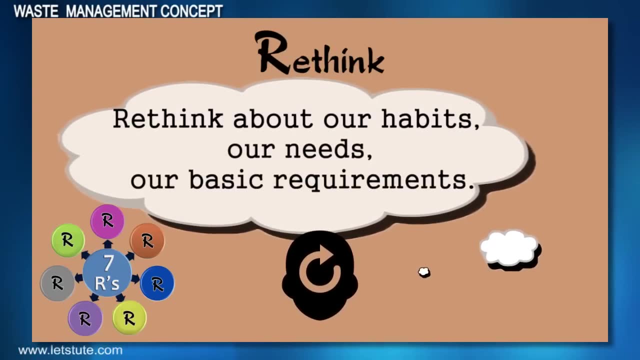 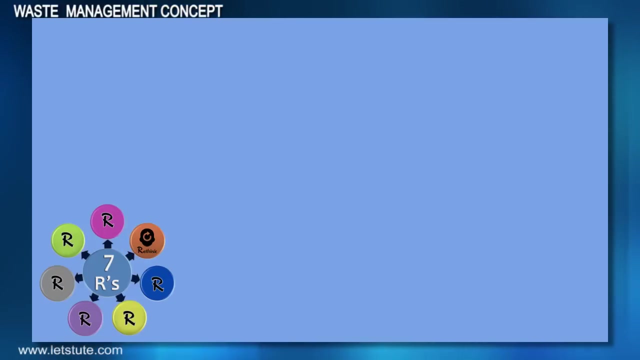 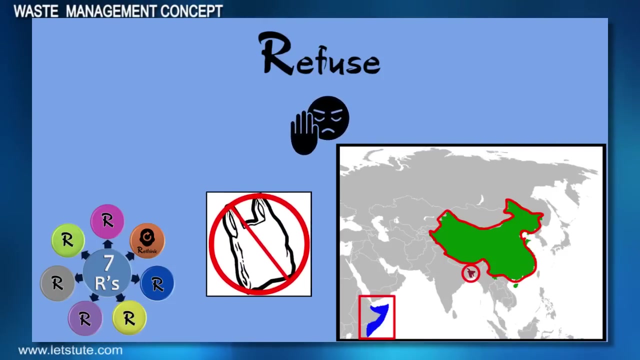 The first R is Rethink. We should rethink about our habits, Our needs or our basic necessities. We must actually think: do I really need this now? The second R is Refuse. Refuse anything that will harm our environment. See, for example, countries like China, Bangladesh, Somalia has refused the use of plastic bag carriers by imposing a ban on it. 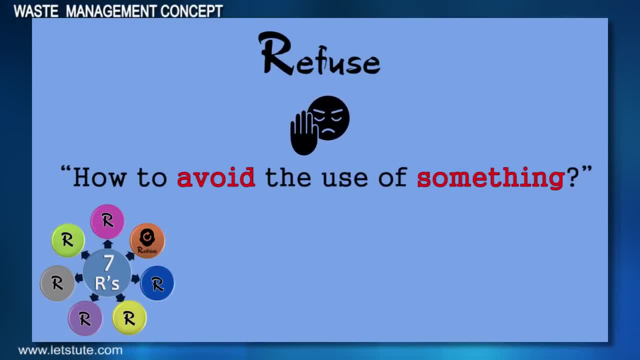 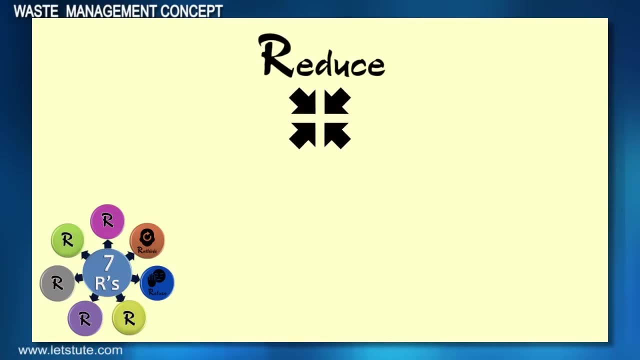 We must think on how to avoid the use of something. The third R is Reduce. This principle focuses on reduction in waste generation. This can be done by repairing, reusing and sharing. Let's think of the ways to reduce the waste formation. 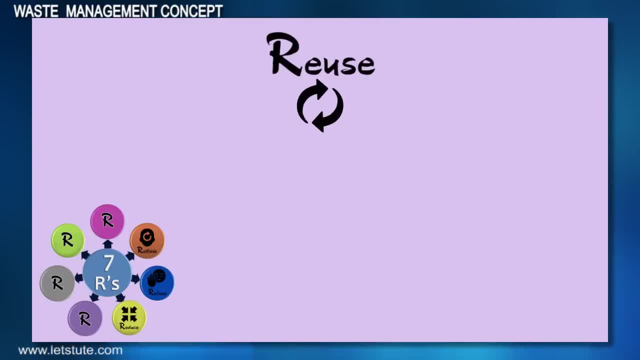 The fourth R is Reuse. Reuse means using something again or more than one time, and thereby reducing the generation of waste. Here we must think of the ways to use the product to its fullest. The fifth R is Recycle. It is reprocessing of unwanted materials into new useful products. 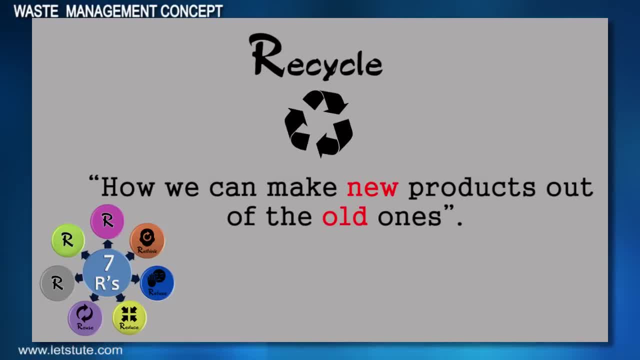 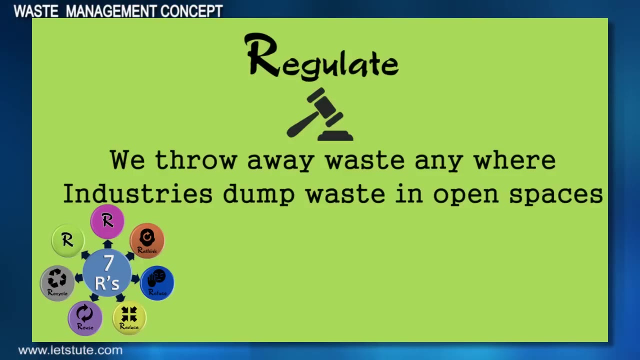 Think of how we can make new products out of the old waste. Think of how we can make new products out of the old waste, products out of the old ones. The sixth R is Regulate. We humans throw away the waste anywhere. Also, many industries release or dump their waste in natural water bodies and open spaces.